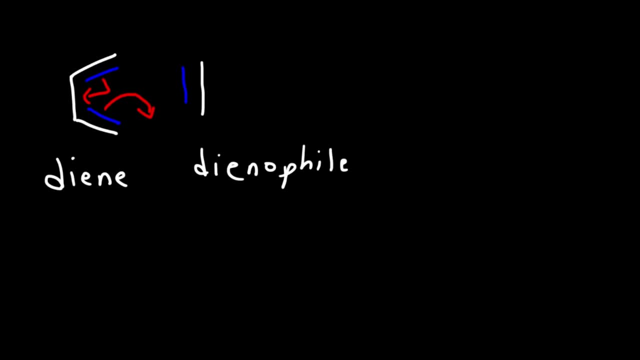 be used to connect these two carbons. Let's call this carbon 1,, 2,, 3,, 4,, 5, 6.. So the second red arrow is used to connect carbons 4 and 5. It creates a sigma bond. 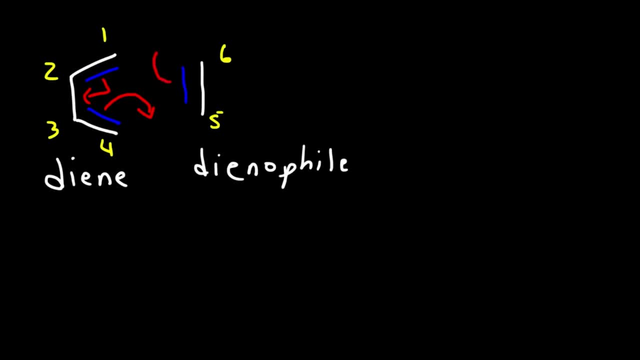 between it And the pi bond between carbons 5 and 6, it's used to create a sigma bond between 1 and 6. And so this is going to give us cyclohexene. So that's a basic introduction into the Diels-Alder reaction. Now let's go over some other. 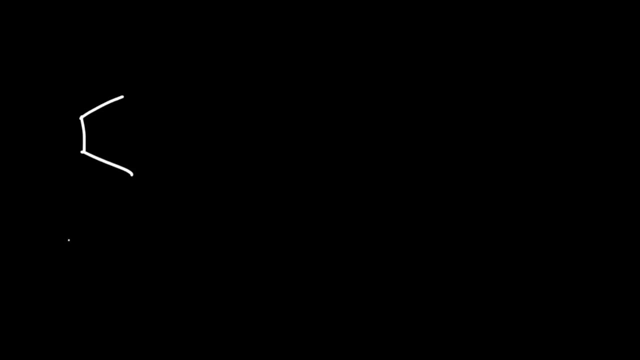 examples. So let's say we have a diene that has two methyl groups. A methyl group is an electron donating group. It's a weak electron donating group but it makes the diene more nucleophilic And we're going to add an electron withdrawing group to the dienophile. So 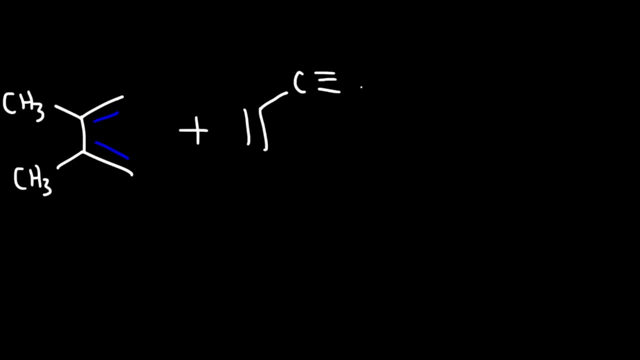 let's use cyanide, Cyan A cyano group. The electron withdrawing groups makes the dienophile more electrophilic and thus more reactive in the Diels-Alder reaction. So you need an electron donating group to enhance the diene. But 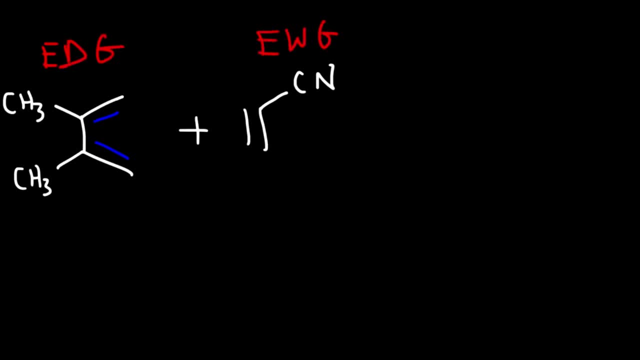 you need to use an electron withdrawing group to enhance the strength of the dienophile, so then these two will react in the same manner, and so we're going to get this product. so let's call this carbon one, two, three, four, five and six. so on carbon two, we have a methyl group. 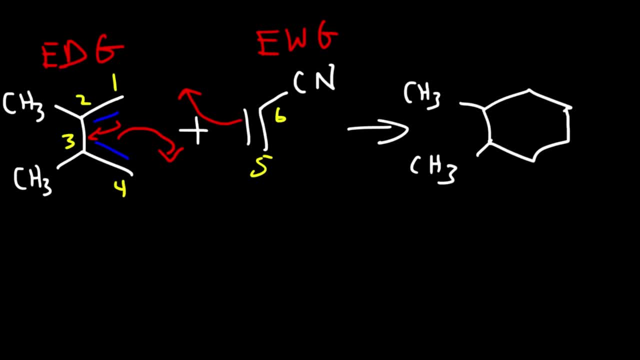 and on carbon three and between two and three, we're going to have a double bond. so this is one, two, three, four, five and six. on carbon six we have a CN group. so this is the product for this reaction. now let's try another example. so once 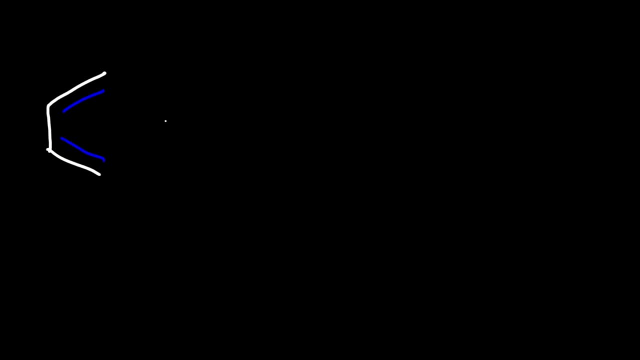 again, we have a 1,3-butadiene in its S-cis conformation and let's react it with this molecule. so go ahead and pause the video and predict the major product of this reaction. so the mechanism is going to be the same, it's not going to change, and so 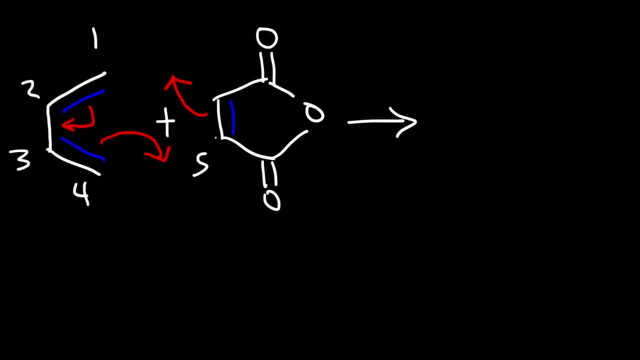 this is going to be carbon one, two, three, four, five and six. so let's start with our six membered ring, and attached to carbon six we have a carbonyl group which is attached to oxygen, and on 5 we also have another carbonyl group. and as 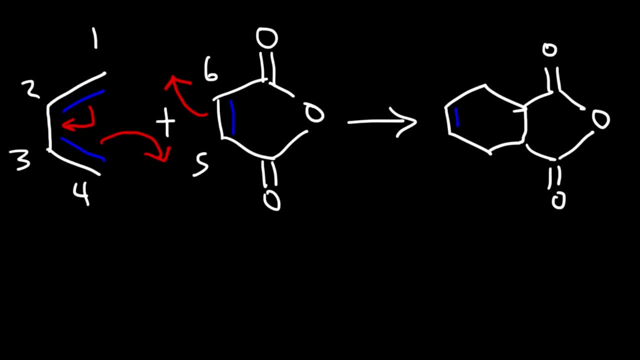 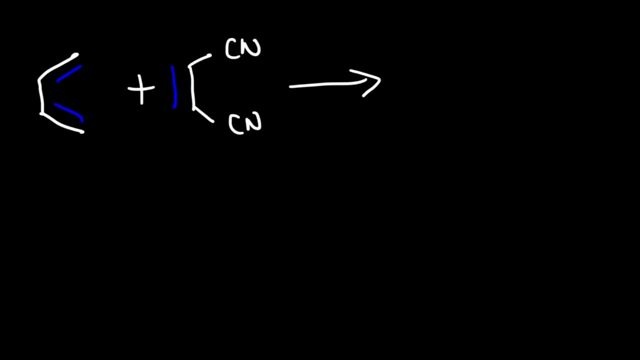 major product will be in this reaction, So the mechanism will be the same. We're still going to get a 6-carbon ring, but notice that the CN groups are on the same side, So when we draw a final product, they should still be cis with. 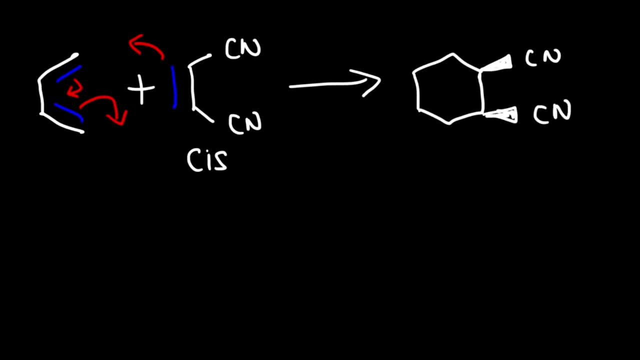 respect to each other. So this is one way in which we can draw the final product. We can also draw it like this as well. In fact, these two products are identical. Notice that we have an internal plane of symmetry. So therefore these two products are meso compounds. So in this reaction, 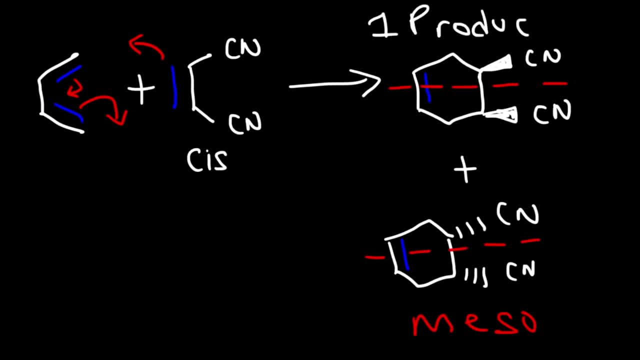 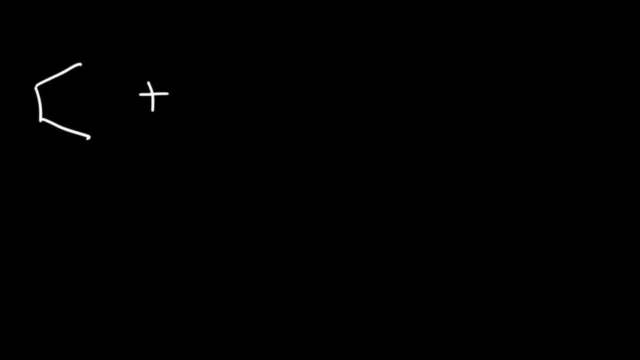 we only get one product as our answer. Now let's try another example. So this time we're going to use a trans alkene, as our dienophile Go ahead and predict the major product for this reaction. So the two carboxylic acid groups have to be on opposite sides with respect to 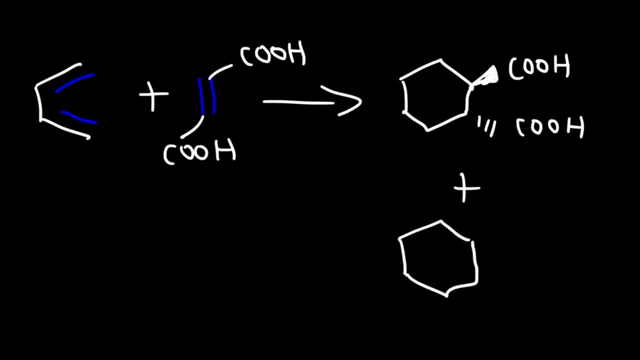 each other, So we can get that compound, plus we can get its enantiomer. So in this case we're going to get a mixture of two different products, both of which are trans. We no longer have an internal plane of symmetry, because this is on the 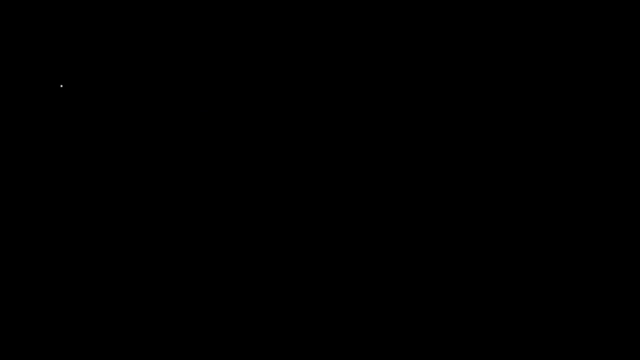 wedge and that's on the dash. Now, in the next example, we're going to react 1,3-butadiene with a dienophile. that is a triple bond as opposed to a double bond. So what kind of product are we going to get in this example? So we're still going to get a six-membered. 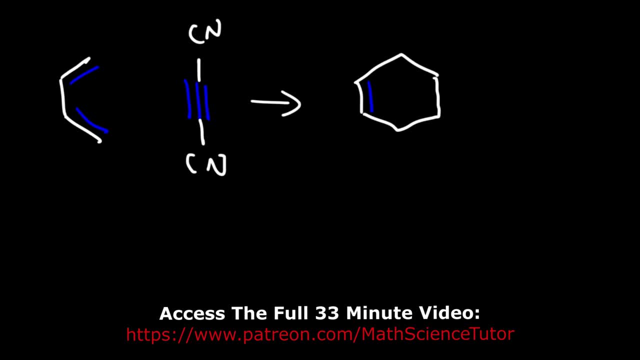 ring and we're going to have a double bond between carbons 2 and 3. Now, attached to carbon 6, we have a CN group and also on 5.. Now, in this reaction, the triple bond is going to go down to a double bond. So we're going to 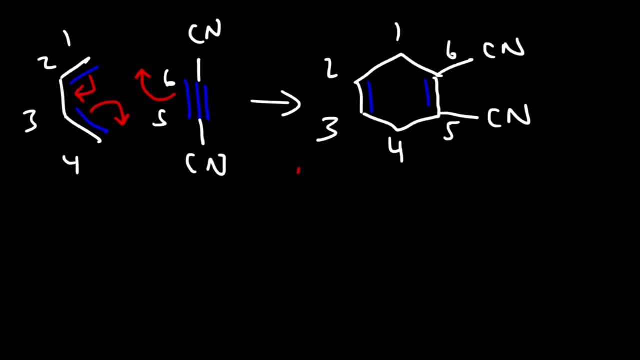 have a double bond between 5 and 6.. So this is the major product for this reaction. Go ahead and try this problem. What is the major product? So on the left we have our diene, On the right a dienophile. But notice, the dienophile has a left side and a right side, So the diene 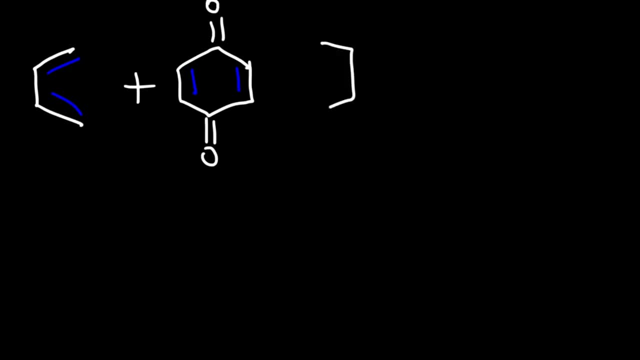 can react on both sides, So it can react on the right side as well, which is what's going to happen. So we're going to get a six-membered ring on the left side and on the right side, So we're going to have a total of three rings. 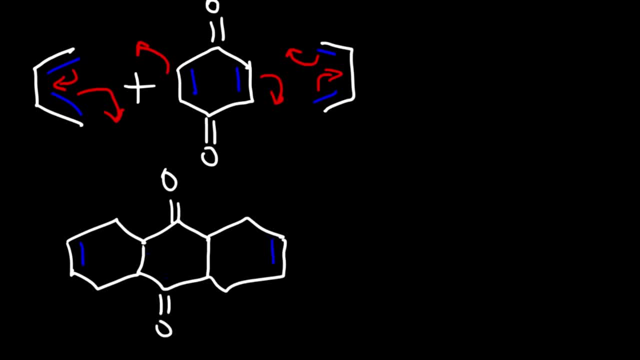 And so this is going to be the final answer for this reaction. Now, what should you do if you have a diene that is already inside of a ring? So here we have cyclopentadiene and we're going to react it with a dienophile. 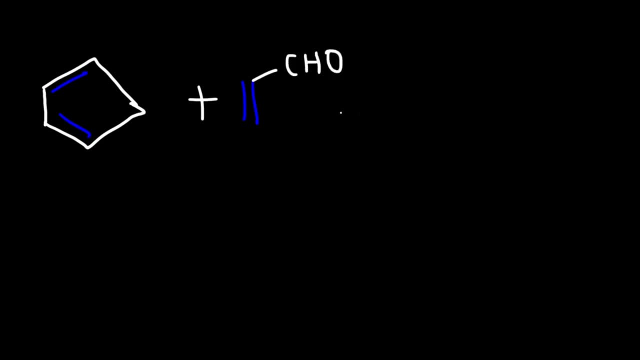 that has an aldehyde function. What is the major product for this reaction? So if you have a diene that's part of a ring in a Diels-Alde reaction, you're going to get another ring, And so you're going to get a bicyclic compound. This is 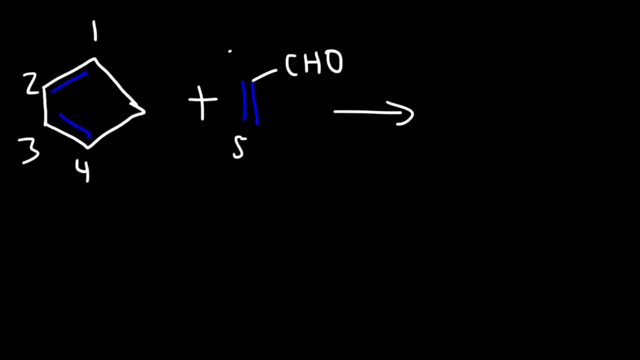 carbon: 1,, 2,, 3,, 4,, 5,, 6.. So I'm going to draw the 6-carbon ring like this. So this is 1,, 2,, 3,, 4,, 5, and 6.. So I'm going to draw the 6-carbon ring like this. So this is 1,, 2,, 3,, 4,, 5, and 6.. So I'm going to draw the 6-carbon ring like this. So this is 1,, 2,, 3,, 4,, 5, and 6.. 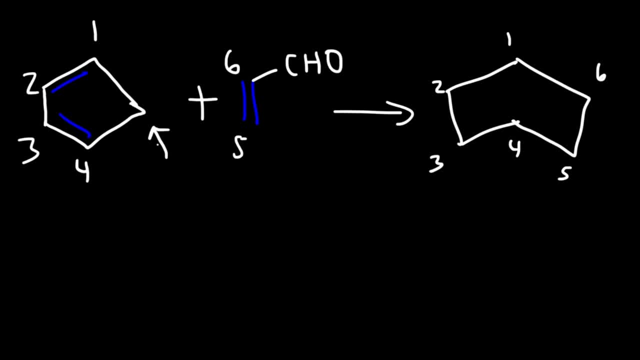 Now notice that we have a methylene group, or CH2 group, attached to 1 and 4.. So in the final product you can put that here. So that's the CH2 group there. Now, attached to carbon 6, we have a CHO group. Now, because I'm running out of space, I'm 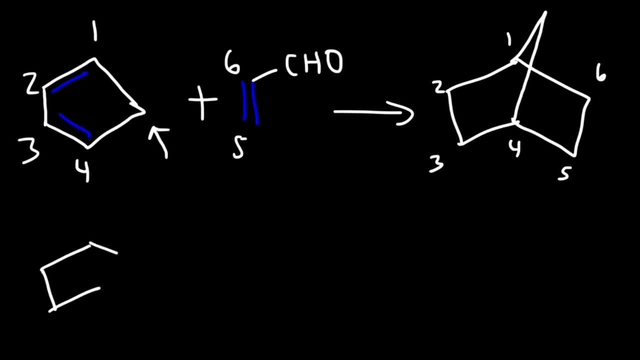 going to redraw that molecule at the bottom. Now, don't forget, though, we still need to put a double bond. Now, the CHO group. we can draw it like this: This is the exo product. or we can write it like this: where it's going down? 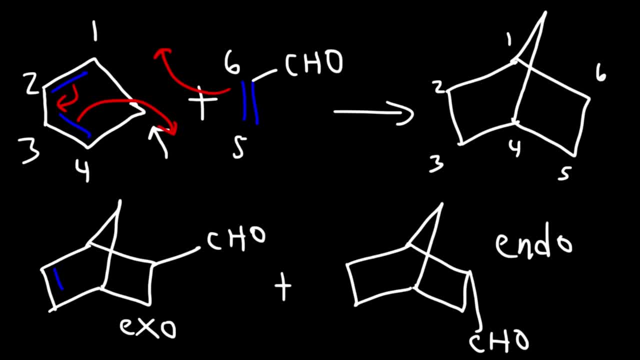 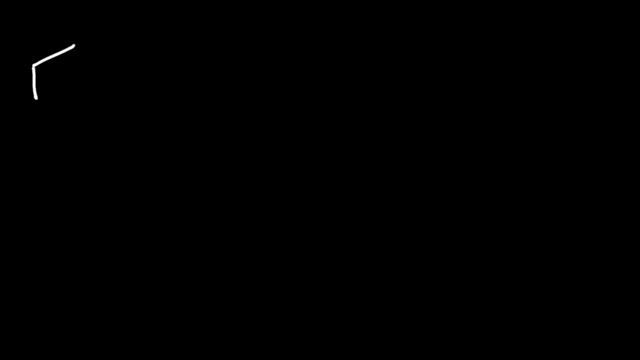 And so that is the endo product. What you need to know is that the endo product is the major product, And so this is going to be the answer. Now let's try another similar example. So this time, instead of having a 5-carbon ring, our diene is going to be inside of a.